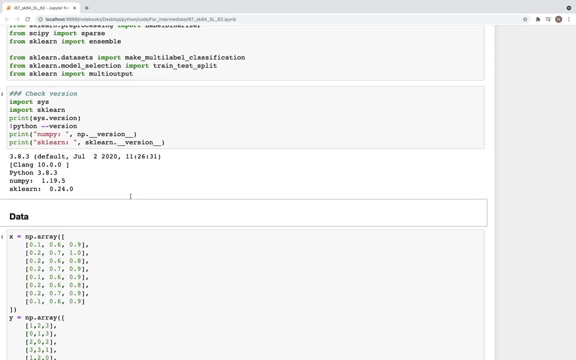 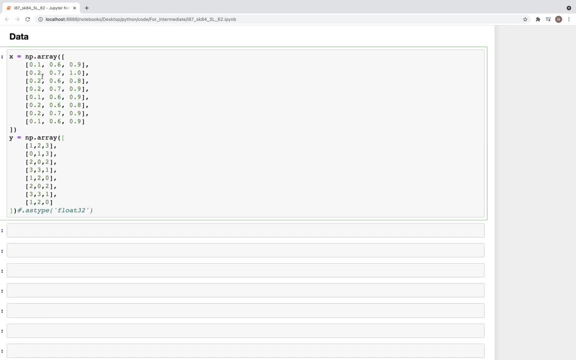 So let's run this and these are the versions that I'm using. Now for data, we'll use this same data set, so this would be our input: features by column, so one, two and three features. and then we have multi, so targets. we have y, which is one, two and three, so we have three different targets, and we'll use this- x and y. but 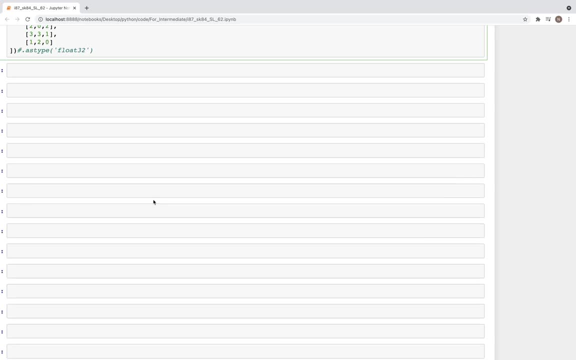 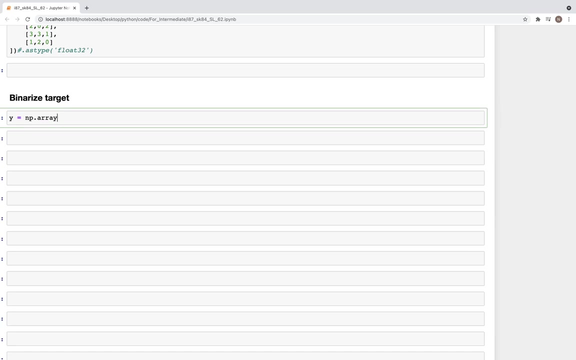 before we do that, for example, to show how to binarize, we'll use a different example. so for binarize target, for this, let's create an array. y is equal to np dot array, and this can be the same as what we used in the previous video, which is car truck. 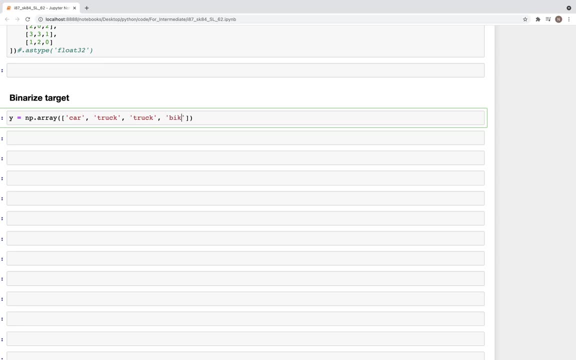 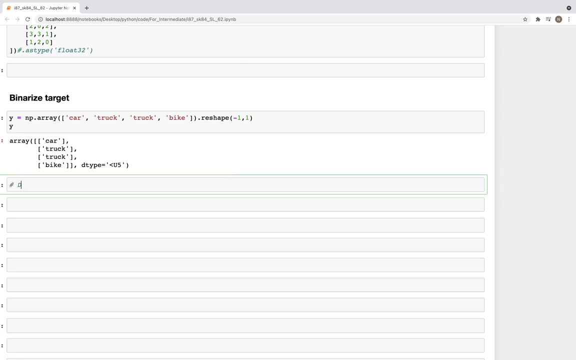 truck. and then, finally, we have a bike, and, if we want to, we can reshape it, but it's not needed. okay, so we have the y. so now we need to binarize this. so what we can do is- so this would be a dense matrix. for this- we can create label. 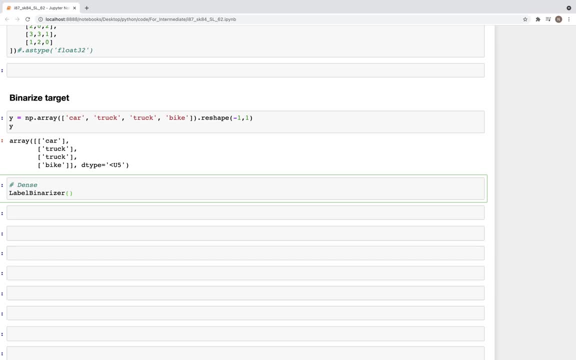 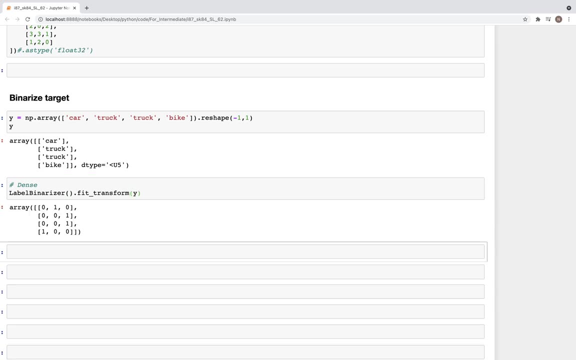 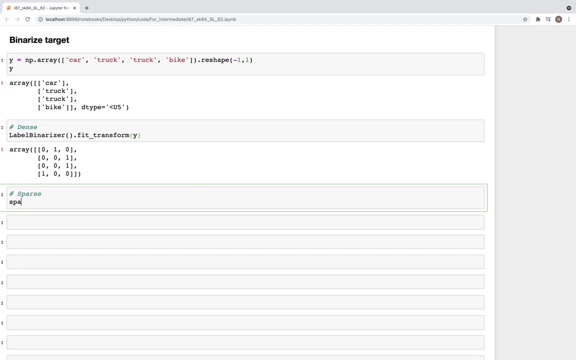 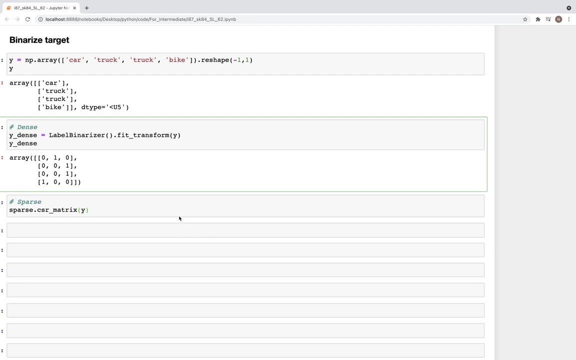 binarizer, and here we can perform fit, transform, y, and so we get this matrix and similar to this. we can get a sparse matrix, also so sparse, which is sparse dot csr matrix y under, so let's call this: y underscore dense is equal to that, so y underscore dense, and then we can use the y underscore dense here. 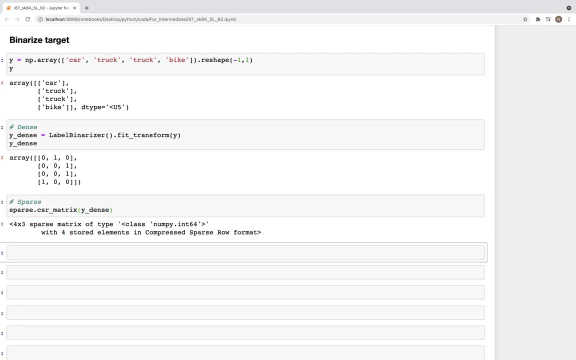 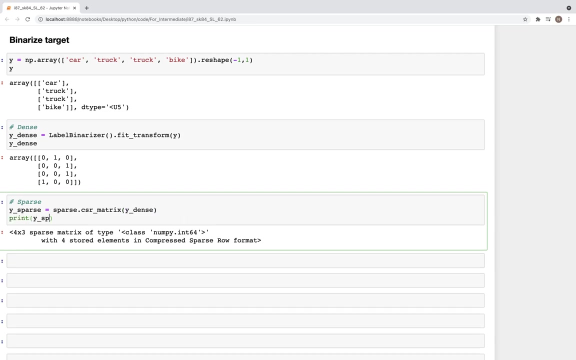 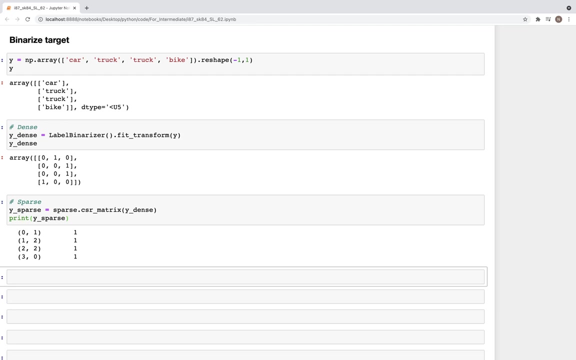 to convert it to: sorry, run those and again. um, so this needs to be printed. so let's put y underscore sparse here and then print y underscore sparse, and here, now we have the output. so so now, as you can see, we have two different variations of the binarized version of the target. 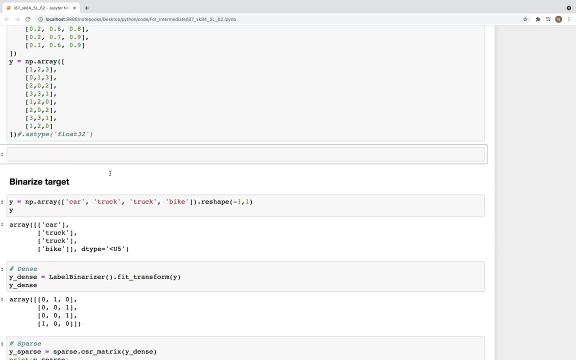 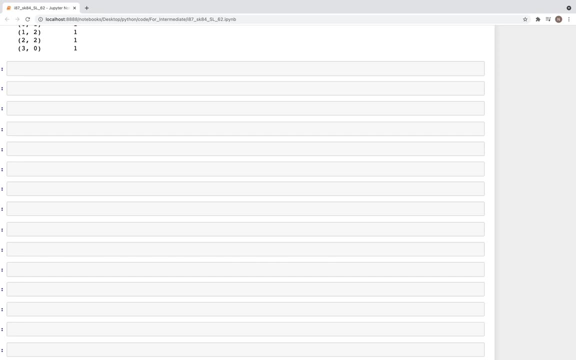 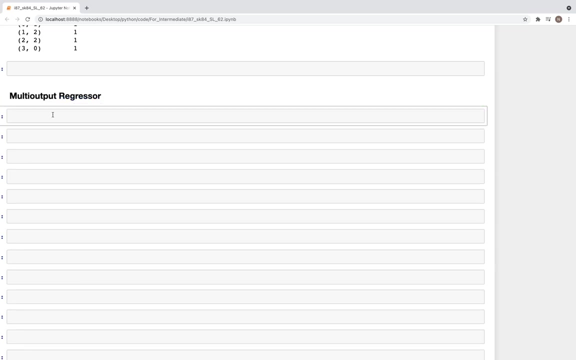 now, with that, i'll go ahead and run this and we can proceed with creating the very first multi output regressor. so multi output output regressor and for this the x and y is what we already have up above. so we'll split that into train and test. 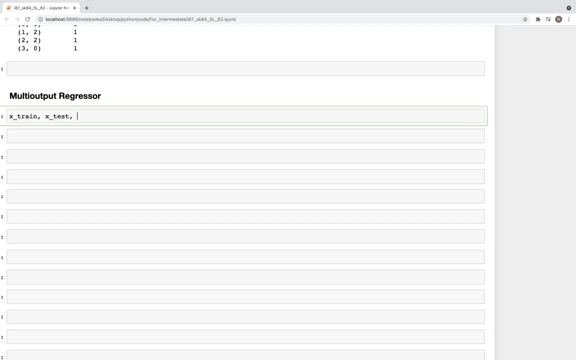 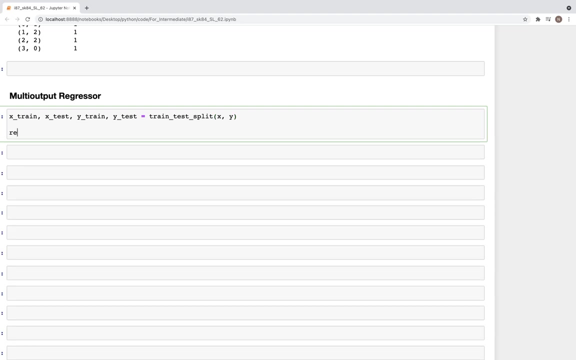 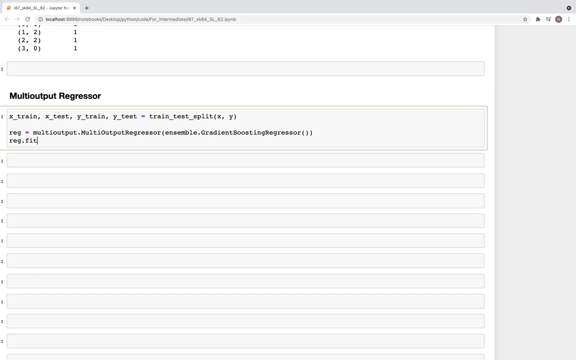 x underscore train x underscore test. y underscore train, y underscore test is equal to train underscore test underscore split x and y and with that we can create the instantiate this variable reg as a multi output dot. multi output regressor and ensemble or gradient is equal to boosting regressor. boost string regressor. 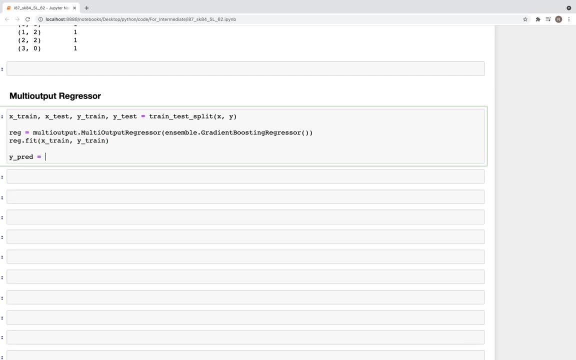 that's what we are using here, and then we can fit this on the x trainick predictäushing and then predict y underscore is equal to regpredict x underscore test. then we can get the matrix as usual. matrix must become 32 Gu흐sorn. 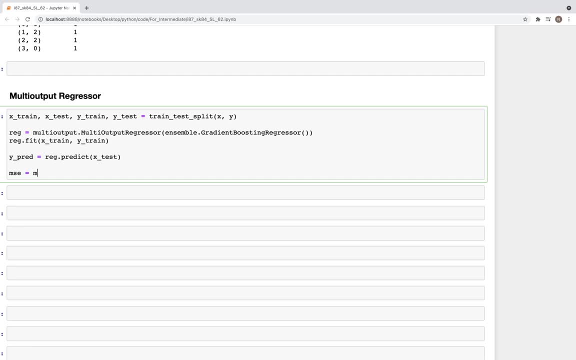 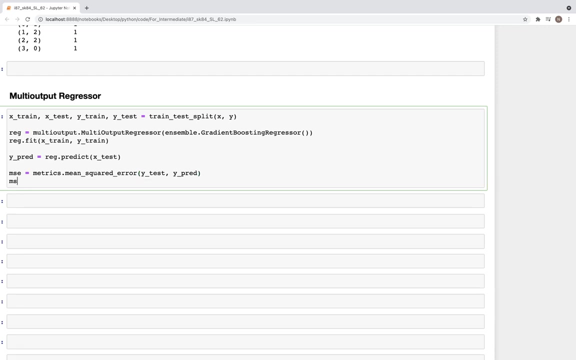 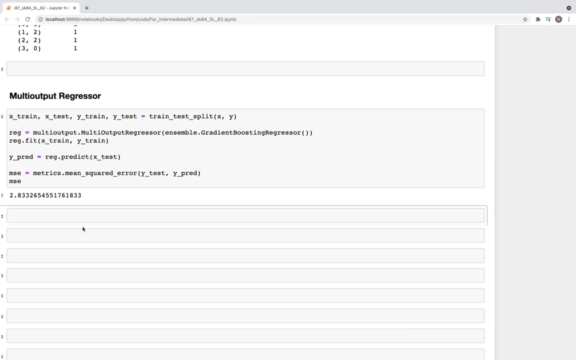 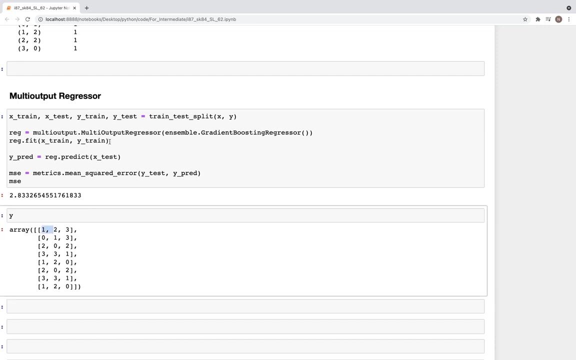 we can get the matrix as usual, matrix, dot mean, underscore squared, underscore error, and here we have y, y underscore test, y underscore pred, and we can get the mac. so that's one implementation of multi output regressor. so here the y that we have has multiple, uh, multiple columns and 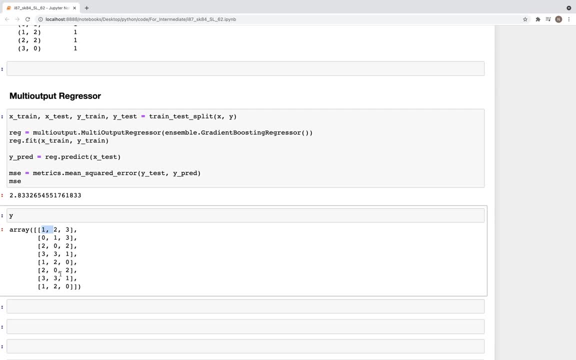 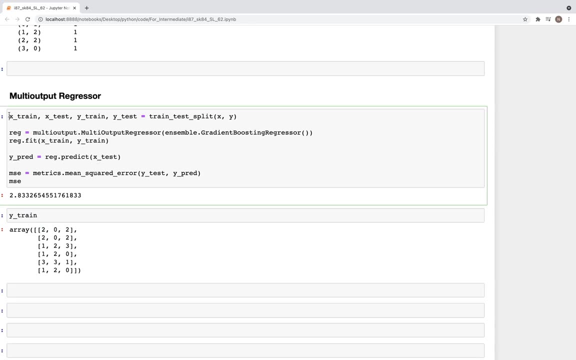 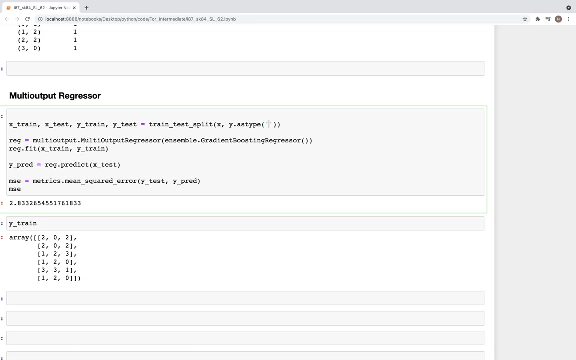 uh. in the previous video i mentioned that these should be floats. if we look at y underscore, train uh it, it is not float. so if we want to, we can convert this to float. so here you can type as type and then type float 32 and then run this. 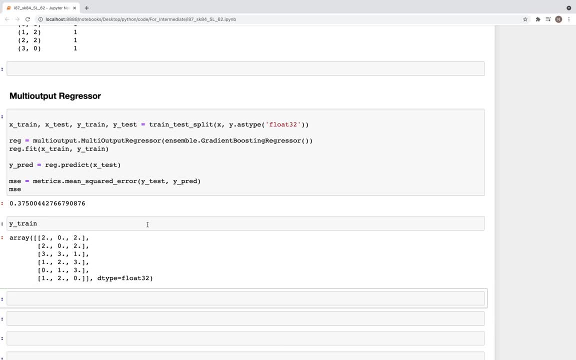 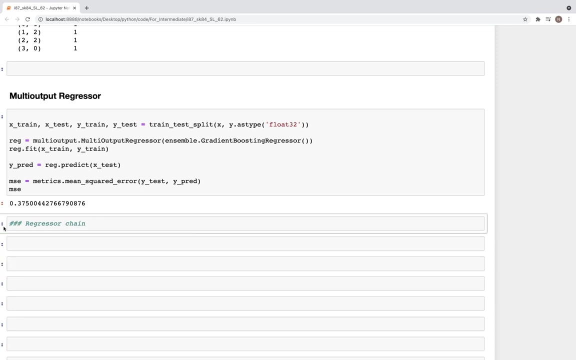 so now we have y. y train is in float format. so that's the mac or the mean squared error we have. now for regressor chain, let's see regressor, regressor chain. for this we'll use again the same data set. let's convert this to markdown, and here what i'm going to. 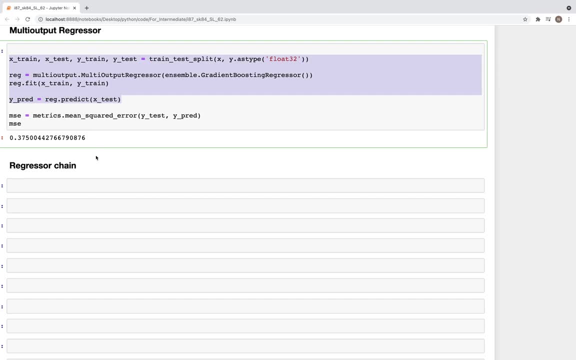 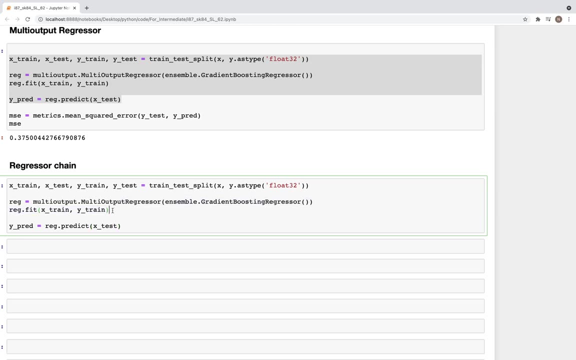 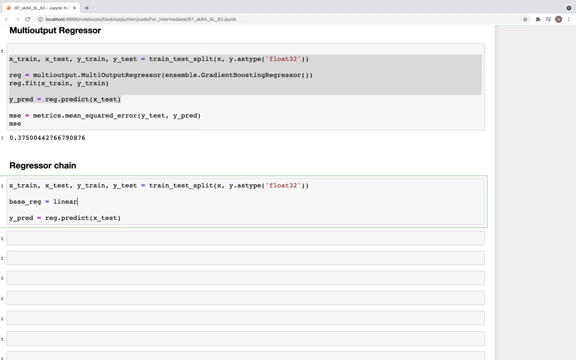 do is i'm going to convert this to markdown. and here what i'm going to do is i'm going to do this do is copy on this entire code from above and the changes would be in this particular part. instead of these, we are going to use variables. let's say: base regressor is equal to linear. 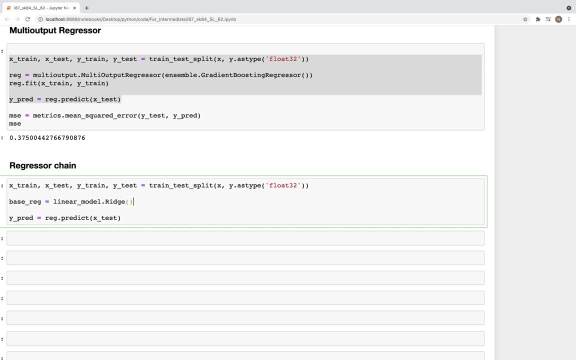 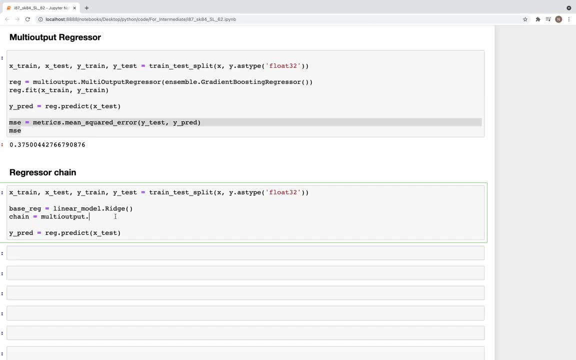 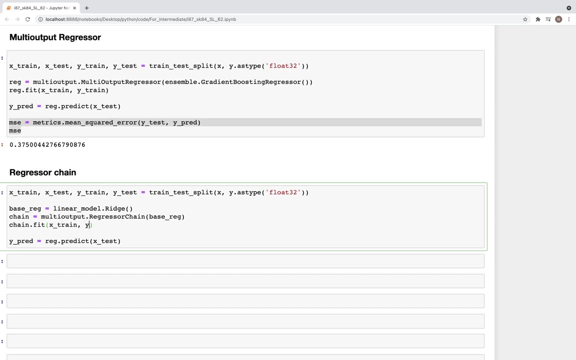 underscore model, dot ridge. so we are using ridge for regression and then for chaining. we have multi output regressor chain base, underscore reg. when we can use the chain fit on x train, y train, x underscore train, y underscore train, then use that to predict and finally we can use the predicted value to get the mac, and so that's the. 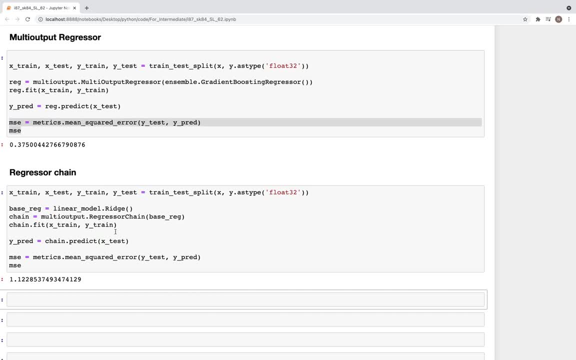 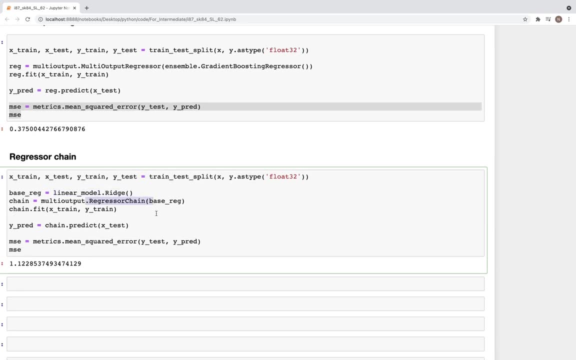 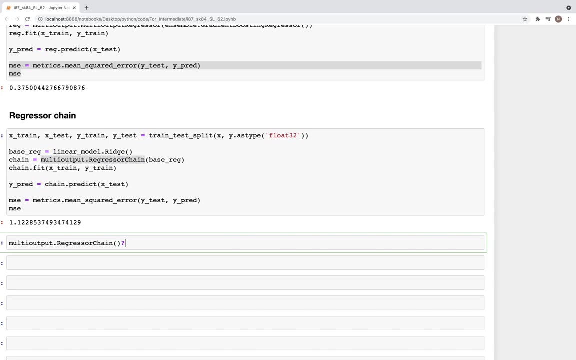 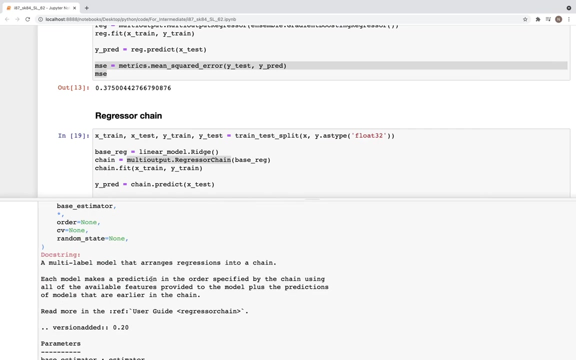 output: mac. so in this case, what we have done is we have used a linear model ridge along with the regression chain, and just to see what regressor chain has as arguments we can look in the docs. so here, as you can see, uh it, it takes a base estimator that we have provided as 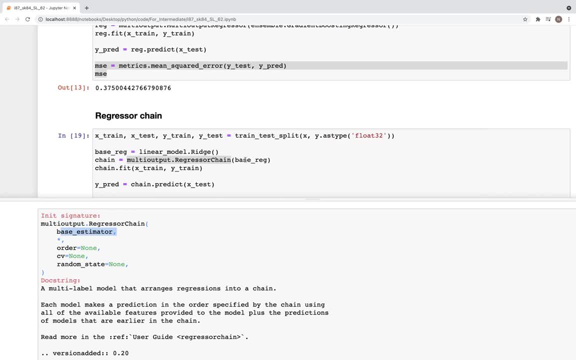 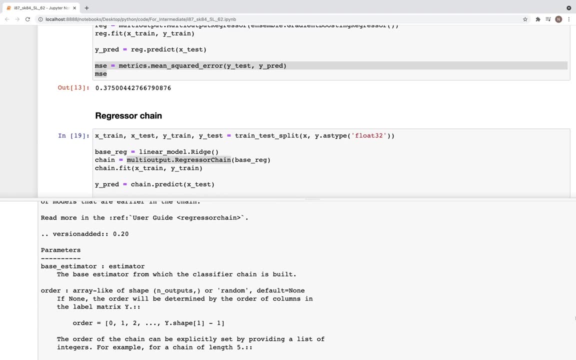 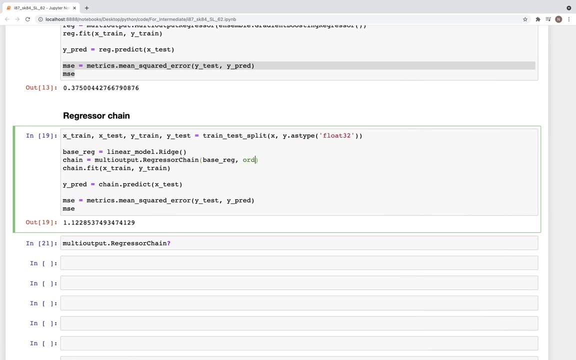 the base underscore reg, and then the order can be anything. so we can also specify the order as random uh in here. so, for example, we could uh specify: order is equal to random and we get that output. now, moving on, let's look at multi output classification. so 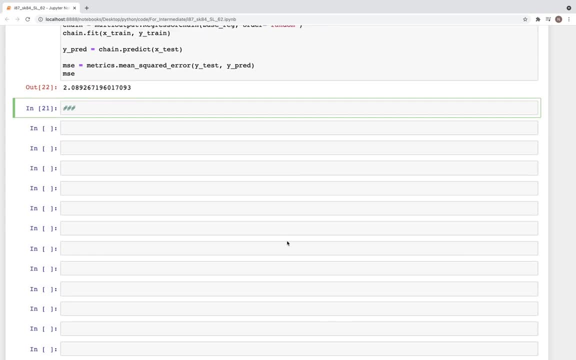 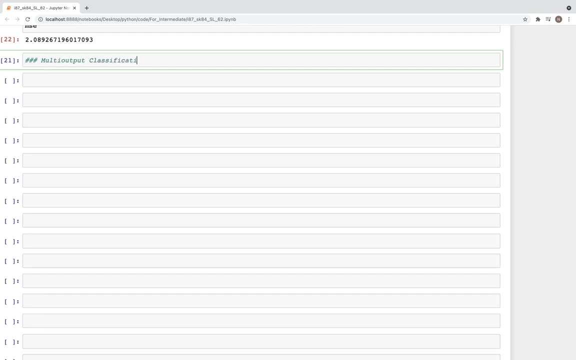 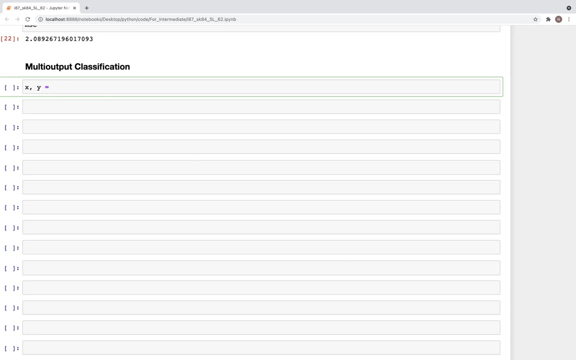 let's move this up and look at multi output classification. we'll create another x and y. x, y is equal to make underscore multi label underscore classification. n underscore samples is equal to 12, n underscore classes is equal to 3 and random underscore state is equal to 0. 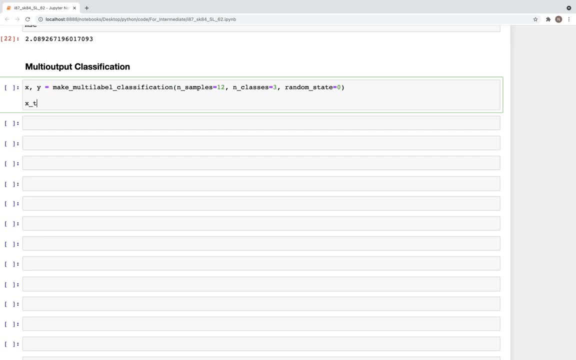 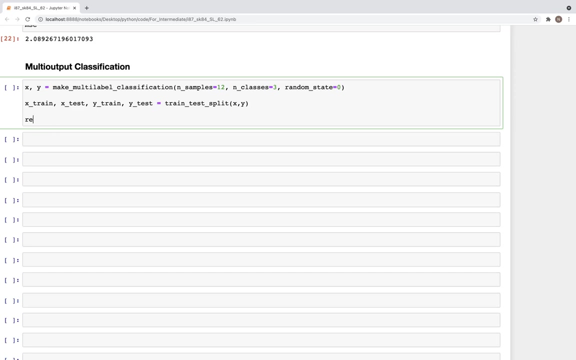 and again we can use the x underscore train, y underscore train- sorry, x underscore test, y underscore train, y underscore test is equal to train underscore test underscore split and this would be x and y and now we have our uh, this classification- so we need clf- is equal to. 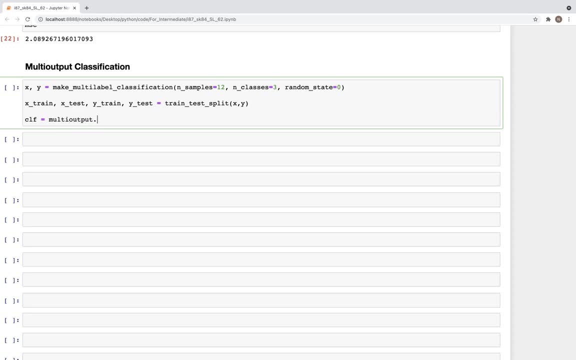 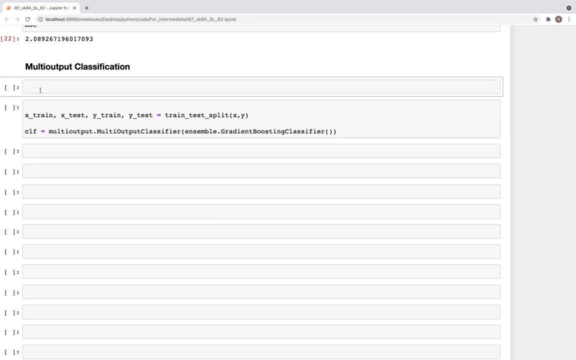 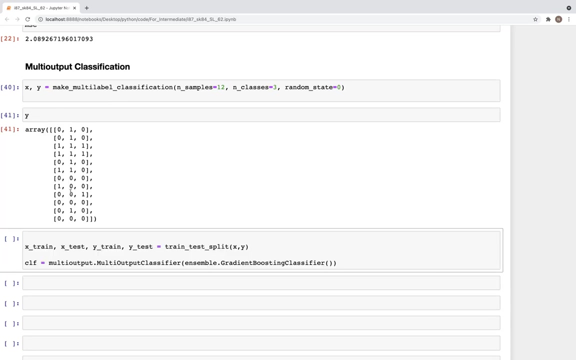 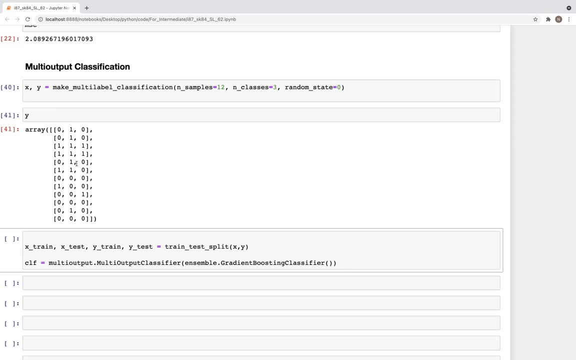 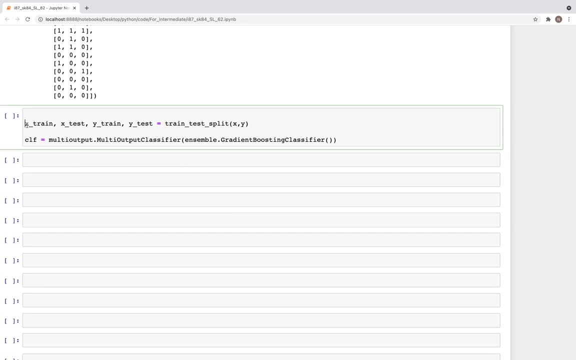 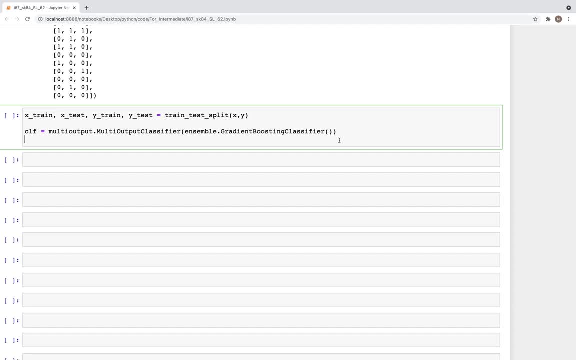 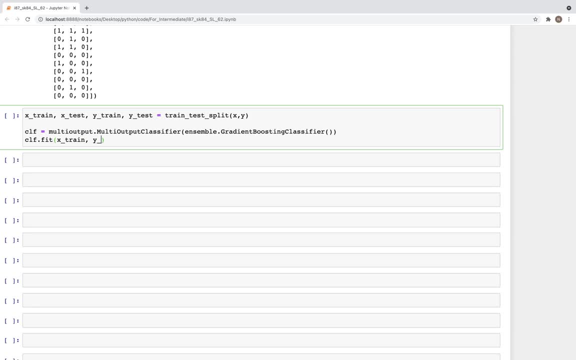 and now we have tlf dot fit. and now we have tlf dot fit on the train x underscore train y, on the train x underscore train y on the train x underscore train y underscore train, underscore train, underscore train, and we can predict so y and we can predict so y. 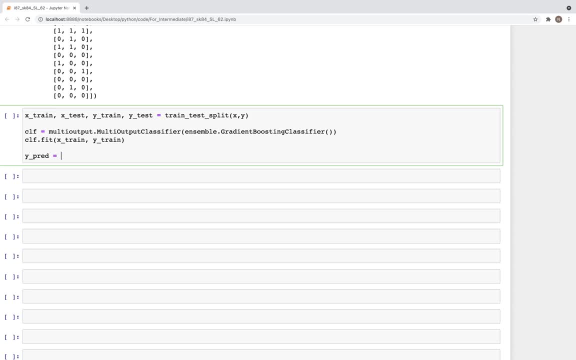 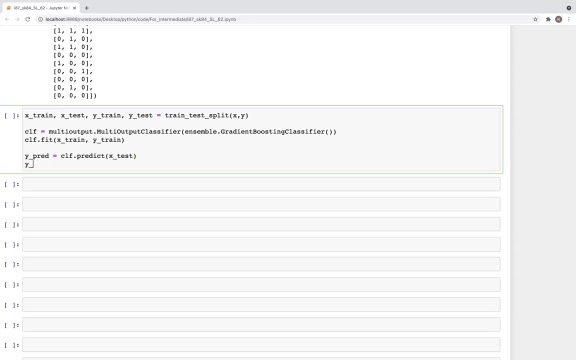 and we can predict so. y underscore thread. underscore thread. underscore thread is equal to, is equal to, is equal to tlf dot predict tlf dot predict tlf dot predict x underscore test. and we have y x underscore test. and we have y x underscore test and we have y underscore pred. 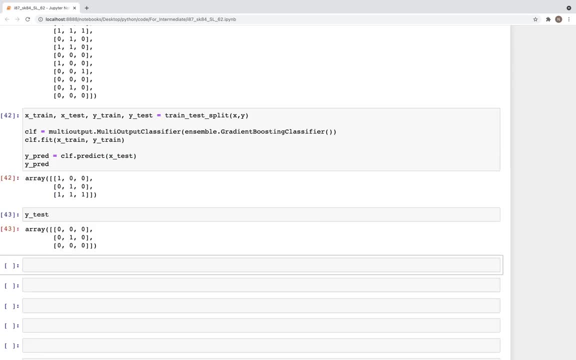 underscore pred. underscore pred there, and this is our y underscore test there, and this is our y underscore test there, and this is our y underscore test. so, so, so, so, these are the. so, these are the. so these are the actual values, and these are the actual values and these are the. 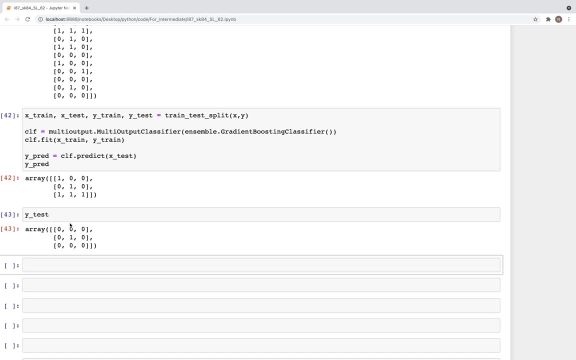 actual values and these are the predicted values. so predicted values, so predicted values. so, uh, this is the small data set, uh, this is the small data set, uh, this is the small data set, and we see that there, and we see that there and we see that there, just this one value was predicted. 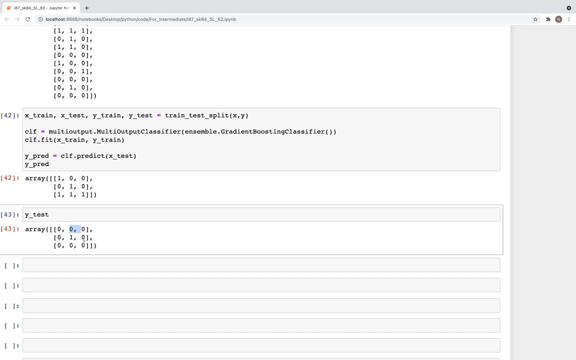 just this one value was predicted. just this one value was predicted correctly. these were correct. so some of correctly. these were correct, so some of correctly. these were correct, so some of them are correct, some of them are not. them are correct, some of them are not. them are correct, some of them are not. now we can use the same data set for the. 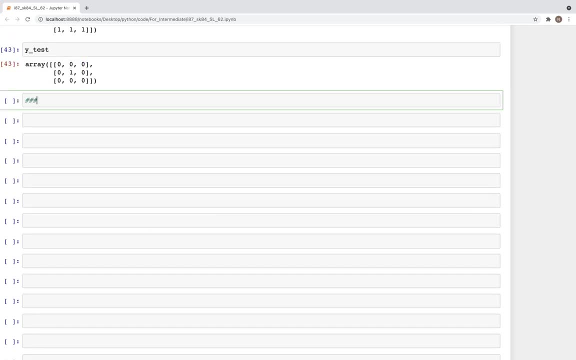 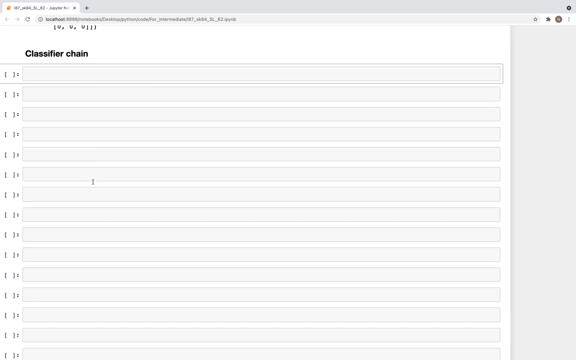 now we can use the same data set for the. now we can use the same data set for the classifier: classifier, classifier chain, chain chain. uh, uh, uh. classifier chain, classifier chain, classifier chain, and, and, and, for this, for this, for this, uh again we can create. uh, again, we can create. 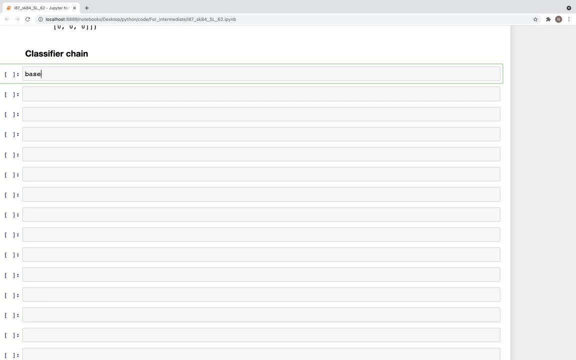 uh, again, we can create. we'll use the same x- y. so here we have: we'll use the same x- y. so here we have: we'll use the same x- y. so here we have: base, underscore, base underscore, base underscore. we'll use linear linear model. we'll use linear linear model. 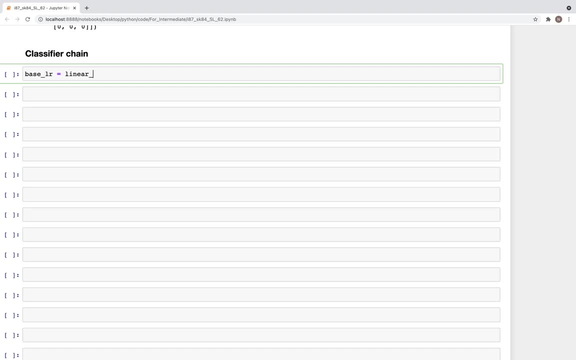 we'll use linear linear model logistic regression. lr is equal to logistic regression. lr is equal to logistic regression. lr is equal to linear underscore. linear underscore, linear underscore. model dot- logistic regression. model dot- logistic regression. model dot- logistic regression, and, and. and. i will use all the default values. then we 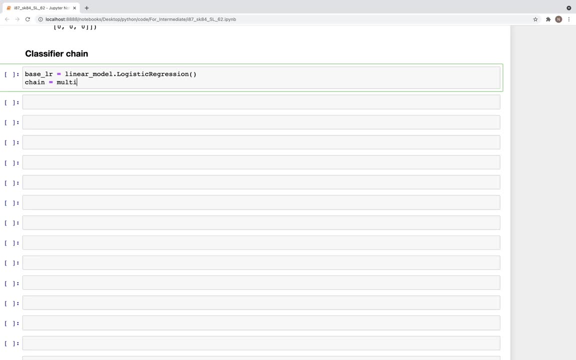 i will use all the default values, then we. i will use all the default values, then we. we can use: chain is equal to. we can use: chain is equal to. we can use: chain is equal to: multi, multi, multi, output, dot, output, dot, output, dot, classifier, classifier, classifier, chain. 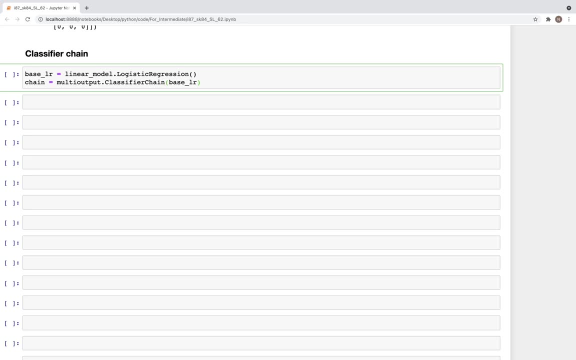 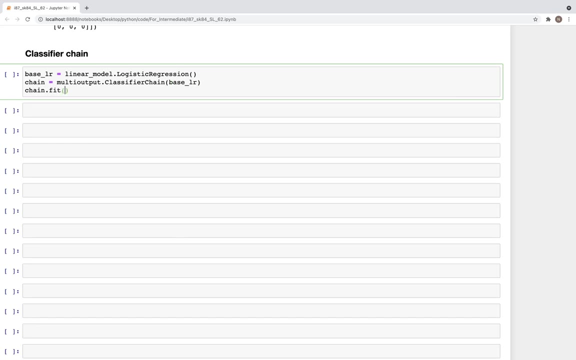 chain chain and this would have base underscore and this would have base underscore and this would have base underscore. logistic regression, logistic regression, logistic regression as an input, as an input, as an input, and we can use the chain to fit on x and we can use the chain to fit on x. 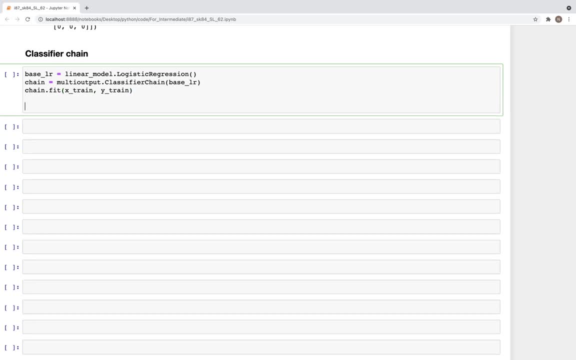 and we can use the chain to fit on x underscore train, underscore train, underscore train, y underscore train and then use the y underscore train and then use the y underscore train and then use the same chain to predict so, same chain to predict so, same chain to predict so. y underscore pred is equal to. 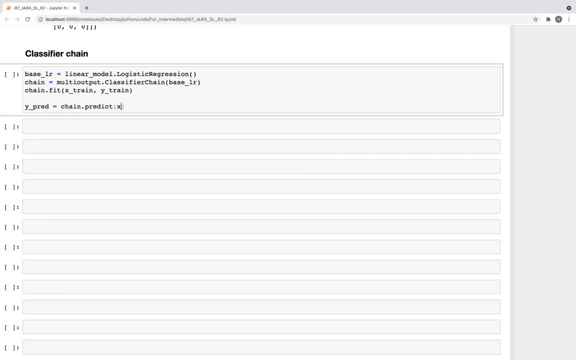 y underscore pred is equal to y underscore pred is equal to chain dot predict x. chain dot predict x. chain dot predict x x underscore test. and now we look at y x underscore test. and now we look at y x underscore test. and now we look at y underscore. 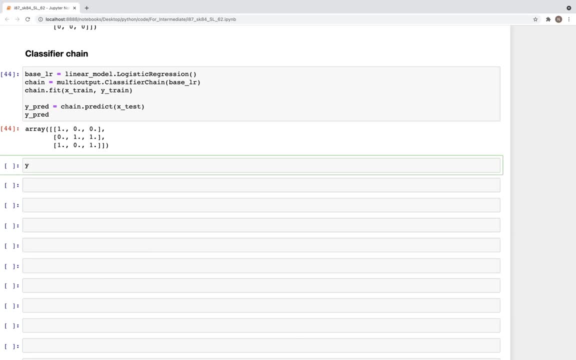 underscore, underscore, pred- so that's the output we get. and pred: so that's the output we get. and pred: so that's the output we get. and y underscore test: that's the original y underscore test. that's the original y underscore test. that's the original data. 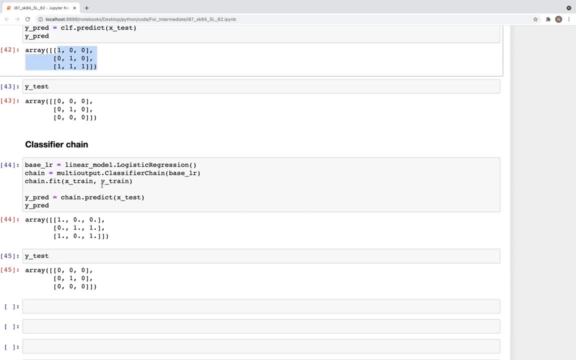 data data. so as we can see in both top this one. so as we can see in both top this one, so as we can see in both top this one and this one, the output is is the same, and this one, the output is is the same. and this one, the output is is the same. but then here we are using 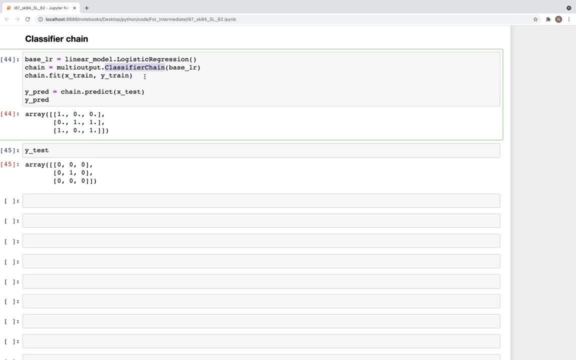 but then here we are using, but then here we are using the classifier chain, the classifier chain, the classifier chain, and here we were not using that, and and here we were not using that, and and here we were not using that. and here we used, here we used. 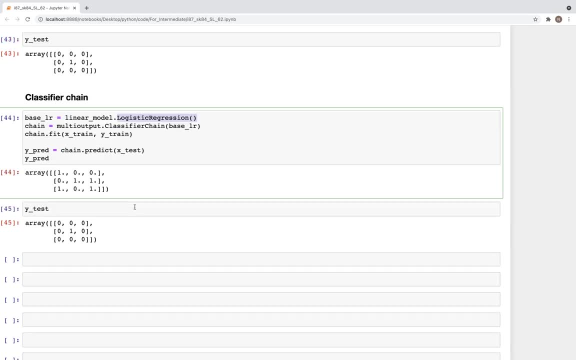 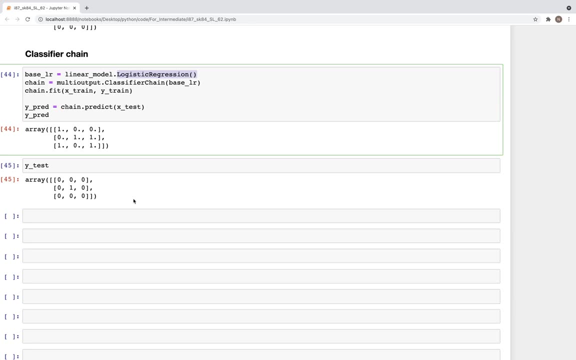 here we used logistic regression, linear model. logistic regression, linear model. logistic regression, linear model upon the classification task, upon the classification task, upon the classification task. so that was it for this video, i hope in. so that was it for this video, i hope in. so that was it for this video. i hope in this and previous video. 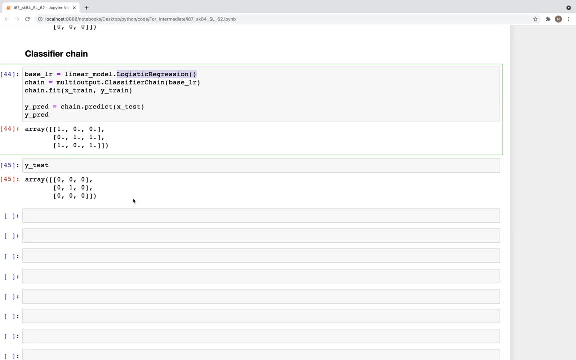 this and previous video. this and previous video, you learn the intuition behind. how to you learn the intuition behind, how to you learn the intuition behind how to uh use, uh, use, uh use these tools in scikit-learn, which is for these tools in scikit-learn, which is for. 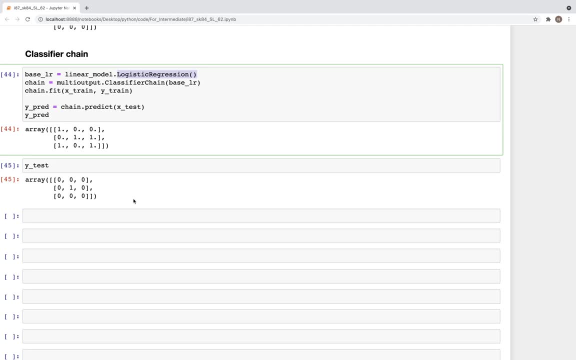 these tools in scikit-learn, which is for multi, multi, multi, multi-class and multi-output, multi-class and multi-output, multi-class and multi-output, classification regression setups. if you classification regression setups, if you classification regression setups, if you have have have more than one targets or if you have, 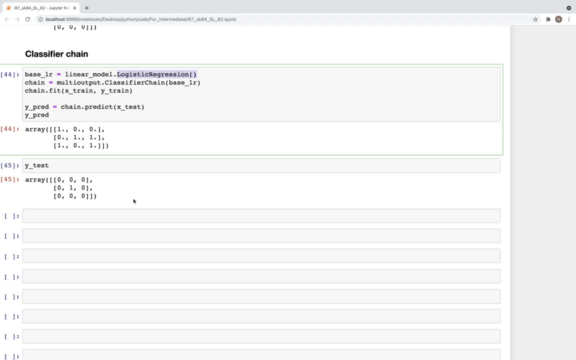 more than one targets, or if you have more than one targets, or if you have a target with more than one classes, a target with more than one classes, a target with more than one classes, you can binarize it into more than one. you can binarize it into more than one. 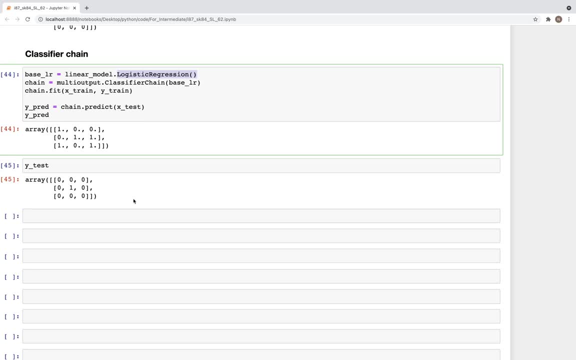 you can binarize it into more than one target, target, target and and use some of these tools to perform. use some of these tools to perform. use some of these tools to perform the predictions, the predictions, the predictions also also also the chaining is. the chaining is. 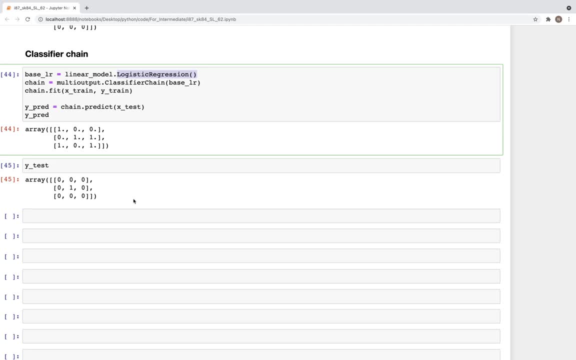 the chaining is very powerful in the sense that, very powerful in the sense that, very powerful in the sense that if you have, if you have, if you have methods that do not natively support methods that do not natively support, methods that do not natively support multiple target outputs, you can chain. 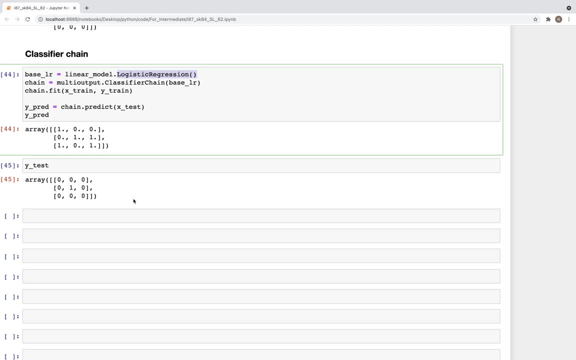 multiple target outputs. you can chain multiple target outputs. you can chain them and use them, here them, and use them, here them and use them here to to to uh, uh, uh, work, work, work to get the multiple targets, to get the multiple targets, to get the multiple targets. uh, work with them. 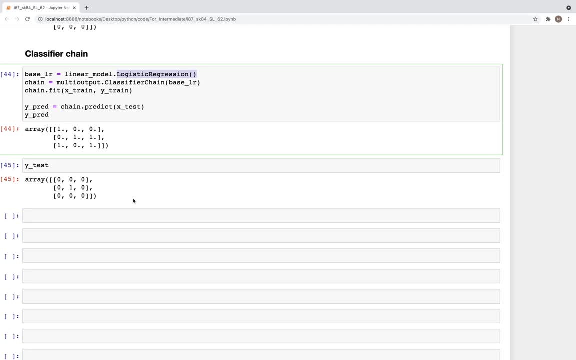 uh, work with them, uh, work with them for for for getting the predict prediction values, for getting the predict prediction values, for getting the predict prediction values. so that was it for this video. so that was it for this video. so that was it for this video. i hope to see all in the next video.